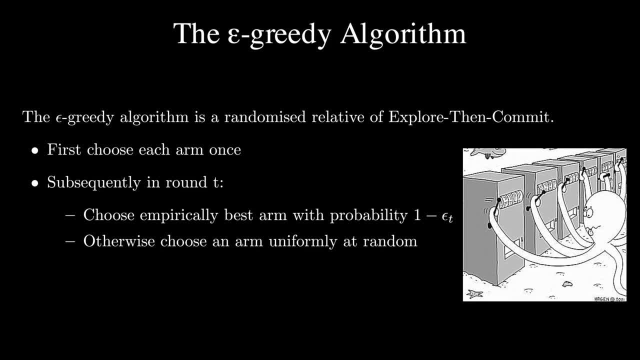 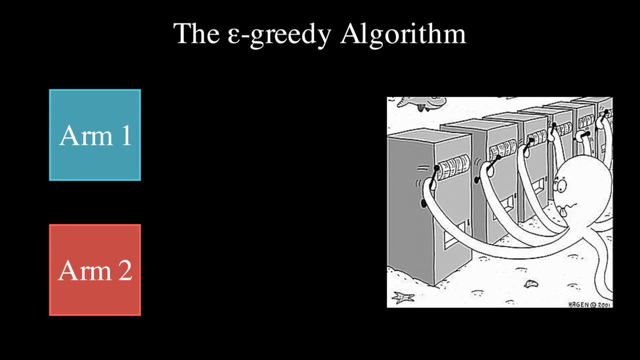 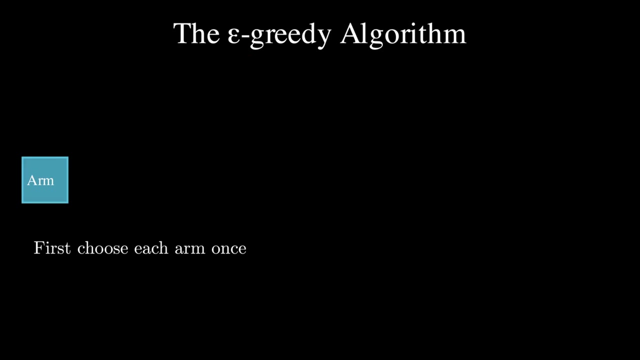 it chooses empirically best arm with probability 1 minus epsilon. Otherwise it chooses an arm uniformly and random. Let's take a look at an example with two arms. Let's assume the rewards for these two arms are one sub-gaucian with a mean of 0.9 and 0.6.. We first play each arm once. At the third round. 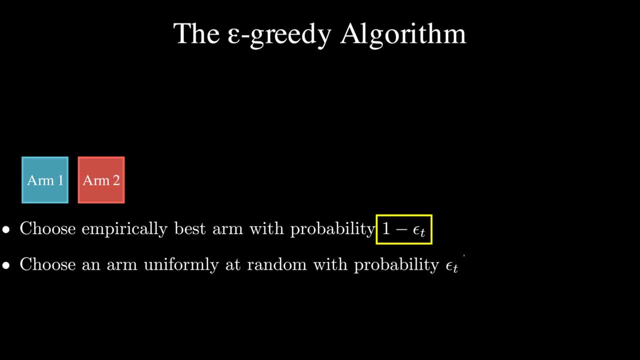 we know that with probability 1 minus epsilon, we choose the empirically best arm And with probability epsilon, we choose an arm at random. In this example, let's assume epsilon 3 equals 1, which means that we have 100% of chance choosing an arm at random. 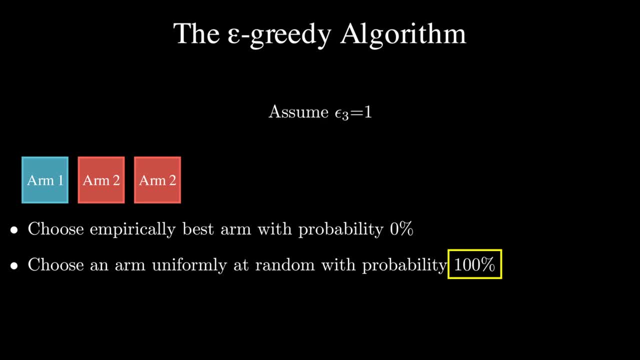 Here in this example, we randomly choose arm 2.. Now assume, at round 4, epsilon 4 is 0.9, which means that with 90% probability we choose an arm at random And 10% probability we choose the best arm. How do we choose? 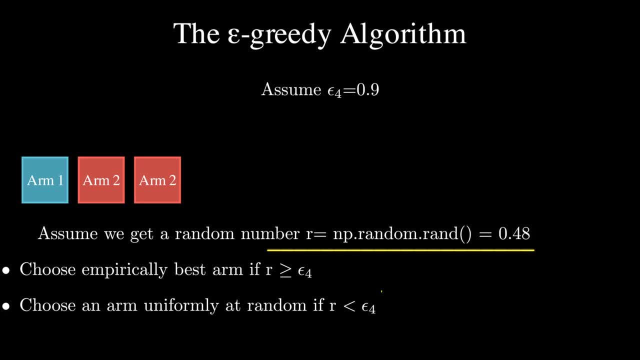 Let's get a random number from this random number generator. Here we get 0.48.. We see that the random number is smaller than epsilon 4.. Thus we choose an arm at random. again, This time we choose arm 1.. 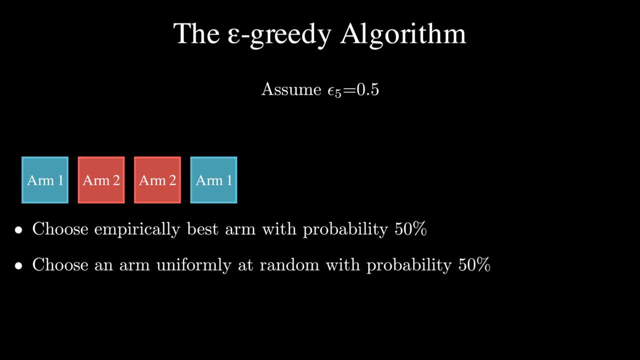 At round 5, assume epsilon 5 is 0.9.. 0.5, which means half of the chance we should choose the best arm. half of the chance we should select an arm at random. Again, we use the random number generator to get a random number- 0.8, which is greater. 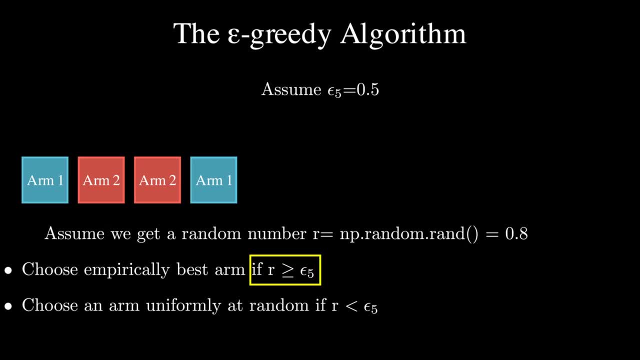 than 0.5,. therefore, this time we need to choose the empirically best arm. How do we find the best arm? Let's assume that in the previous four rounds we played arm 1 gives us a reward of 0.9,. 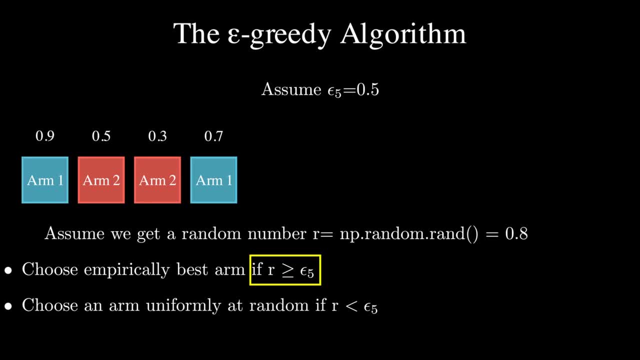 arm 2 gives us 0.5, and then arm 2 gives us 0.3, and then arm 1 gives us 0.7.. The empirical mean estimate for arm 1 is 0.8, and for arm 2 is 0.4..